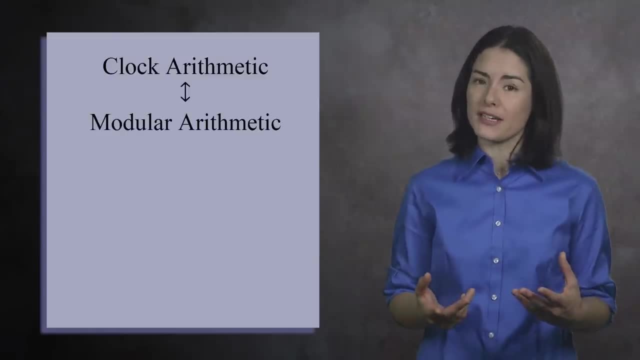 Clock arithmetic is also called modular arithmetic. In the example we just saw, there are seven hours, so we call them the integers mod seven. 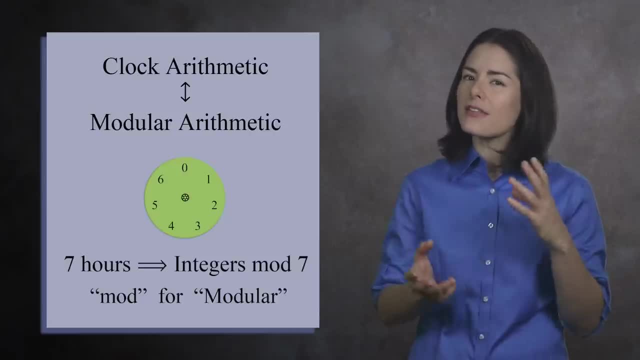 Mod is short for modular. At first glance, you might think this is just an amusing number game, but it has many applications in math and computer science. 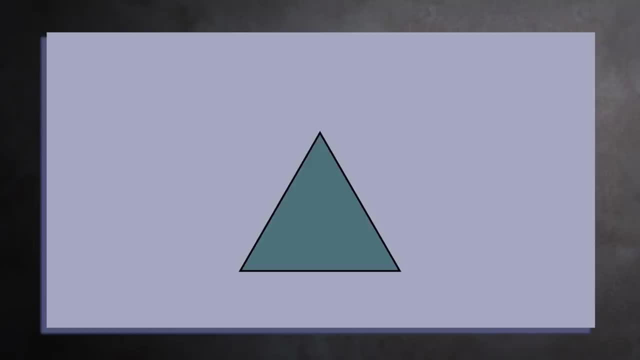 For our next example, let's look at an equilateral triangle. We'll number the three corners one, two, and three. Here's a puzzle. How many different ways can you pick up the triangle, rotate and flip it around, and then set it back down so that it's in the same starting orientation? Hmm? Let's count. 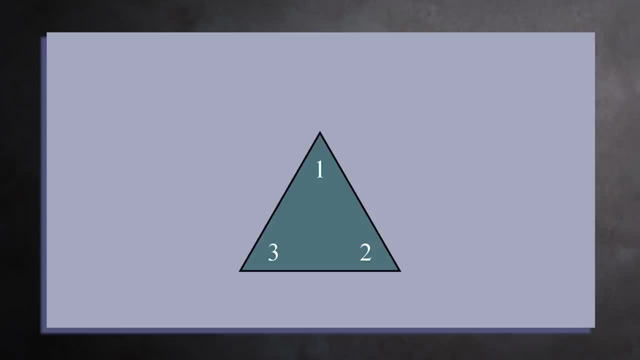 You get the first transformation by picking up the triangle and setting it back down again, unchanged. 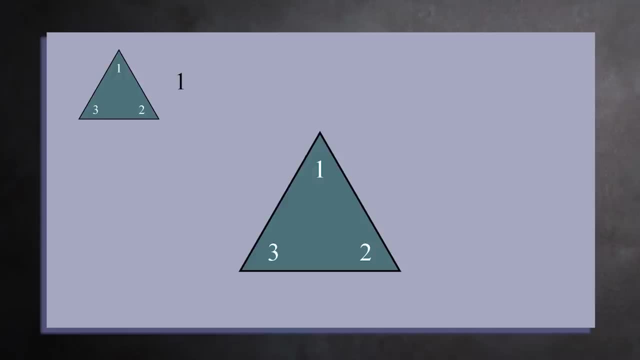 We'll call this transformation one. Let's now find the other ways you can rotate and flip this triangle so that it overlaps itself. 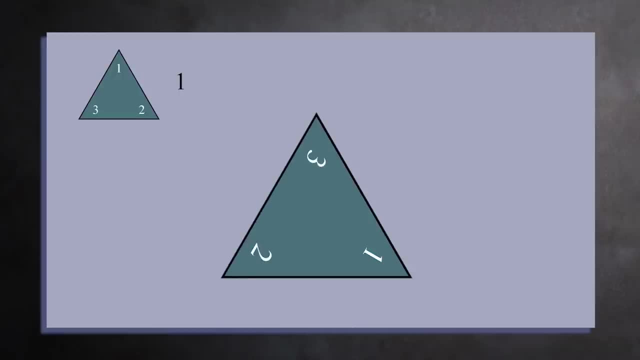 For starters, you can pick up the triangle and rotate it 120 degrees clockwise. This gives you three, one, two. We'll call this transformation R for rotation. If you perform two such rotations, you get two, three, one. 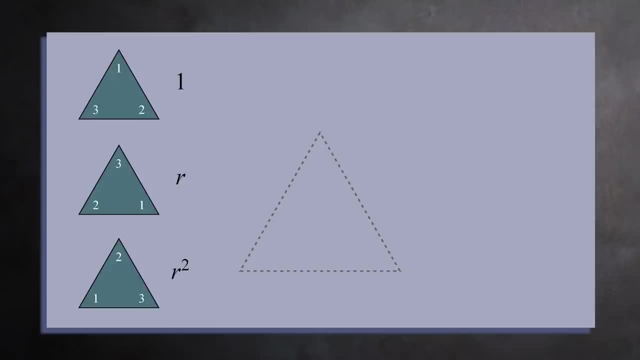 We call this transformation R squared since we applied R twice. And if you do three rotations, you return to the starting position, one, two, three. This means that R cubed equals one. Next, if you pick up the triangle and flip it about the vertical axis, you get one, three, two. We'll call a flip about the axis F for flip. If you flip it twice, you return to the starting position, so F squared equals one. You could also flip, then rotate, which gives two, one, three. And finally, you can flip, then perform two rotations, which gives three, two, one. This covers all possible transformations. 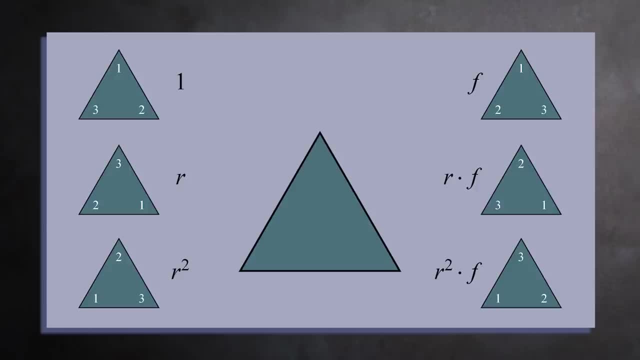 There are six altogether. Notice that there were two basic transformations, a 120-degree rotation, which we called R, and a flip about the vertical axis, which we called F. Aside from the unchanging transformation, each of the transformations are combinations of these two actions. Notice you can multiply any two transformations by first applying one, then the other. In particular, if you multiply any transformation by one, you get the same transformation. This is because one doesn't actually change the triangle. 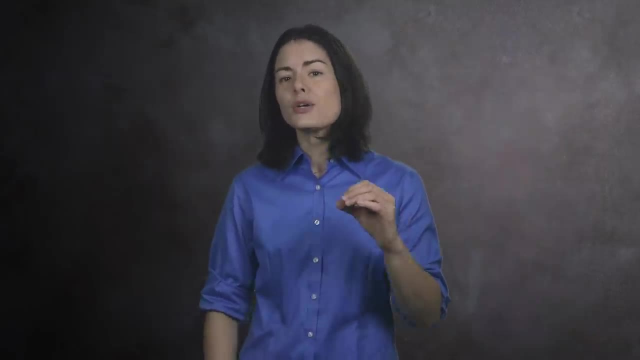 This is one way to study a shape in geometry. Look at all the ways to transform the shape onto itself. These transformations are called symmetries. 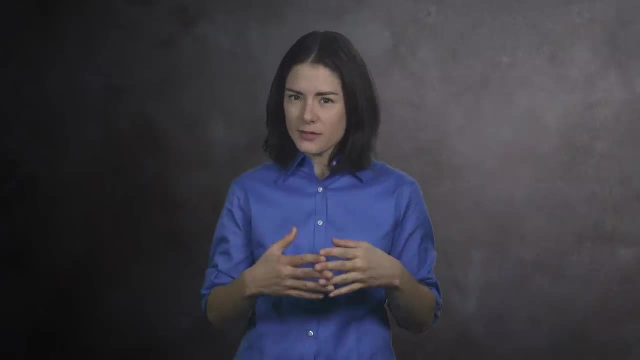 Believe it or not, there is a close relationship between the symmetries of a shape and clock arithmetic. Before we see this connection, let's look at one final example, the integers under addition. 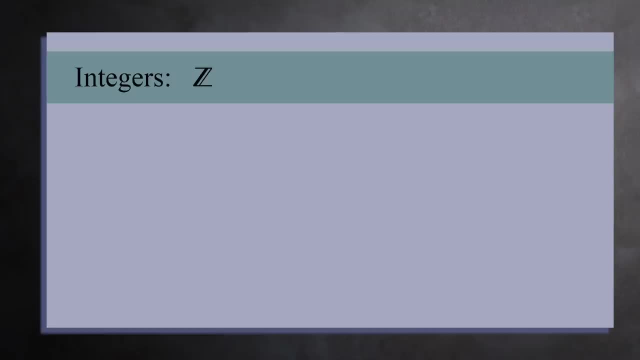 The integers, which we denote by the letter Z with a double stroke, are the set of all whole numbers. Let's look at a few interesting properties of the integers. You can add and subtract any two integers. 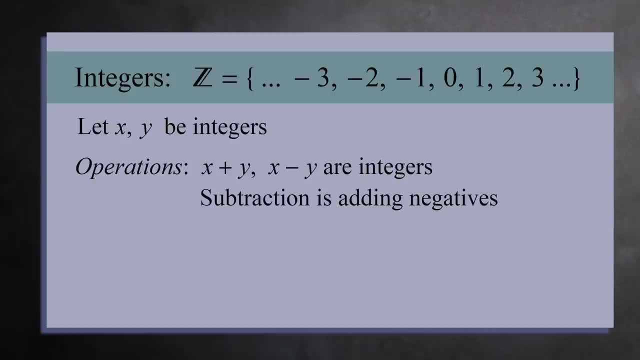 But notice that subtraction is really just adding with negative numbers. For example, 7 minus 11 is the same as 7 plus negative 11, which is negative 4. 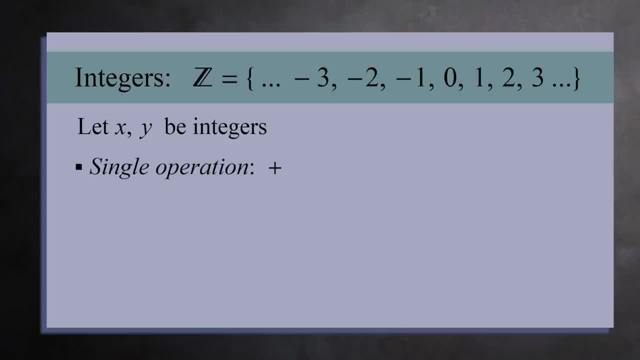 For this reason, it's common to say there's a single operation, addition. If you add any two integers, you get another integer. 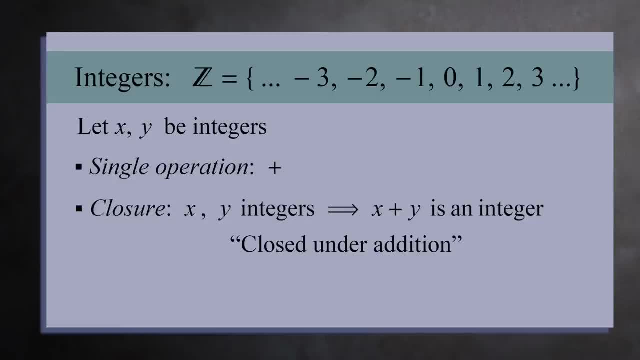 We say the integers are closed under addition. But if you divide one integer by another, you may not get an integer. For example, 3 divided by 5 is 3 fifths, which is not an integer. 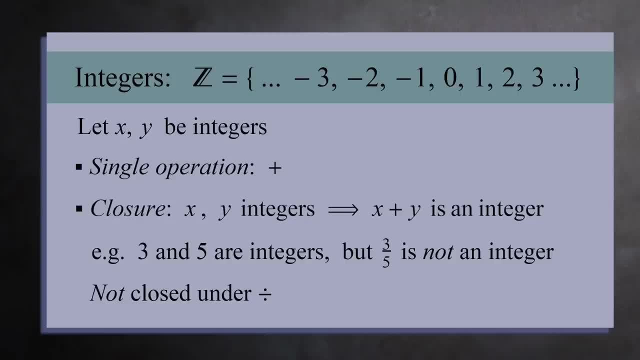 So we say the integers are not closed under division, because when you divide two integers, you may get a number outside the set of integers. 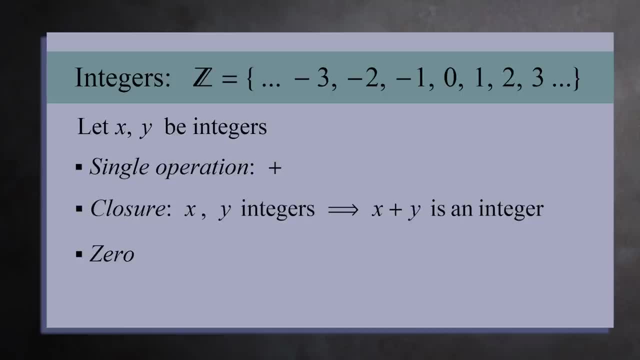 And there's one number which has a unique property, 0. If you add 0 to any integer, you get the same integer. It has no effect when adding. 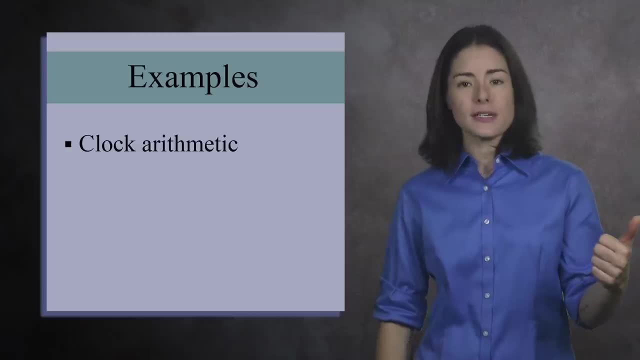 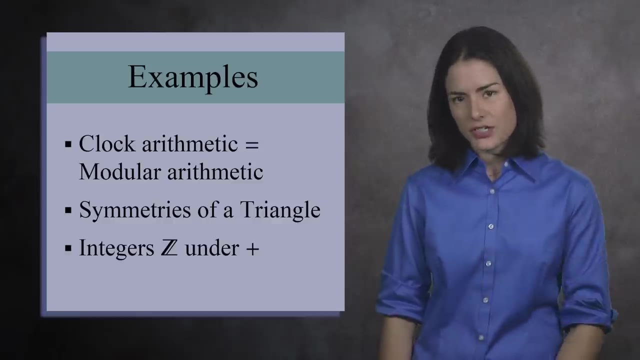 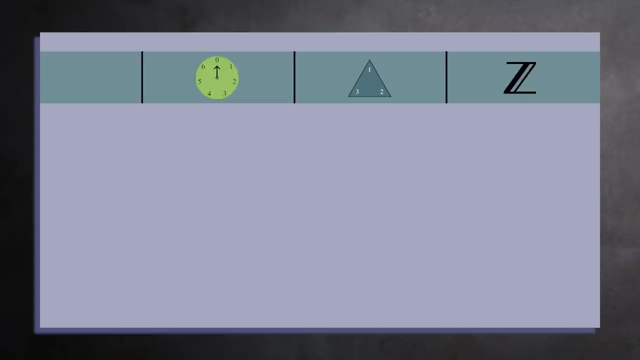 So we've now seen three very different examples. Clock arithmetic, which is more commonly known as modular arithmetic, the symmetries of a triangle, and the integers under addition. Let's now see what these three examples all have in common. To begin, each of these examples have a set of objects which we call elements. For the integers mod 7, the set of elements are the numbers 0 through 6. 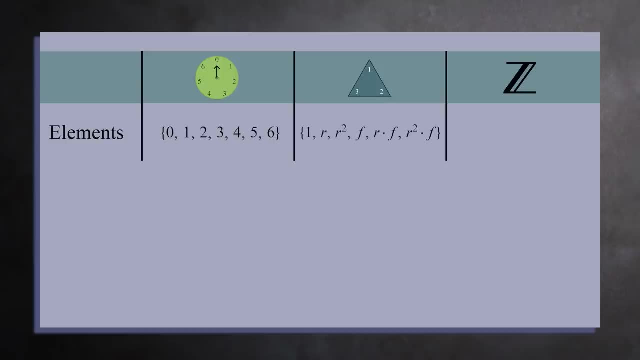 For the triangle example, the set is not the triangle, but the geometric transformations, which we also call symmetries. 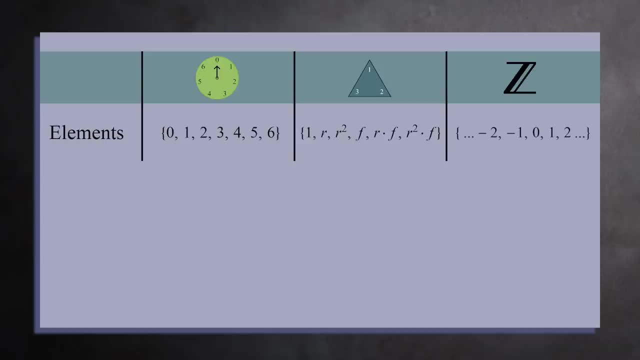 And for the integers, the set is the infinite collection of whole numbers. Next, for each of these sets, there's a way to combine any two elements to get another element in the set. 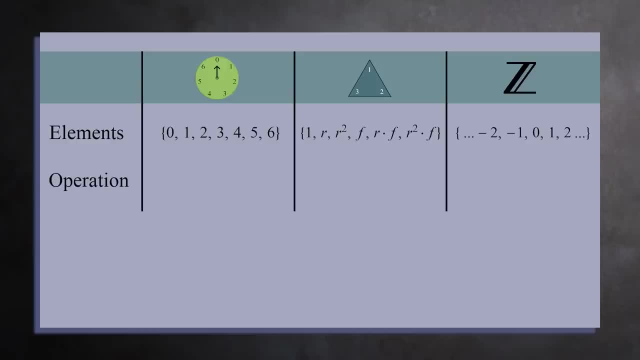 We call this an operation, and we use a symbol to show that we are combining two elements. For the integers, the operation is addition, and the symbol is the plus sign. For the integers mod 7, the operation is also addition. In modular arithmetic, we also use the plus sign, even though addition means something different on a clock. 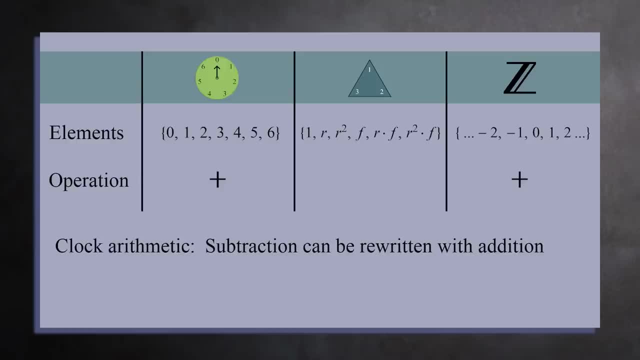 As with the integers, subtraction is redundant. Any subtraction problem can be rewritten as an addition problem. 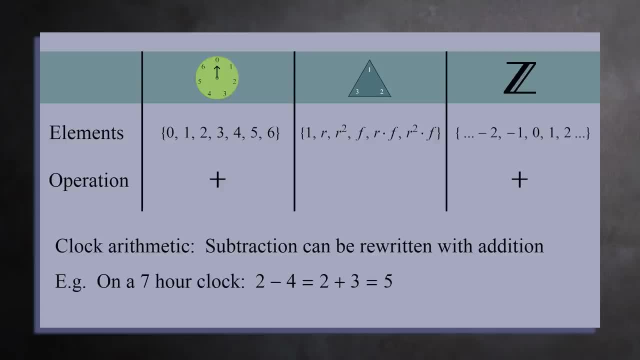 For example, 2 minus 4 is the same as 2 plus 3. 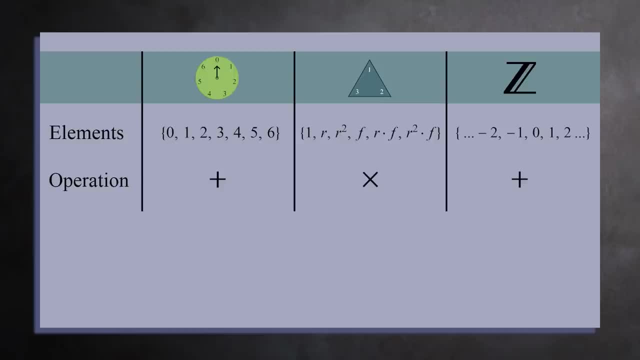 And for the symmetries of a triangle, it's common to use a multiplication symbol. You could use a different symbol if you'd like, but people tend to reuse the addition and multiplication symbols a lot with groups. 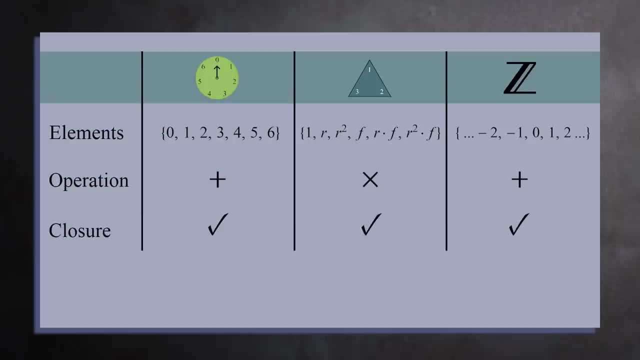 It's also important to remember that each of the three sets are closed under the operation. That is, if you pick any two elements A and B in the set and combine them, you get another element in the set. 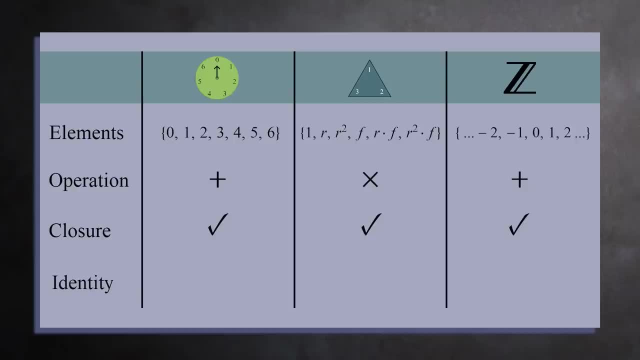 All three structures also have something called an identity element. This is an element that has no effect when combined with other elements. For the integers mod 7, it's 0. If you take any number x on the clock and add 0, you get x. For the triangle, the identity element is the transformation 1. This is a transformation where you pick up the triangle and drop it. You drop it unchanged. If you multiply any transformation y by the transformation 1, you get y. And for the integers, the identity element is also 0. For any integer z, z plus 0 equals z. And 0 plus z equals z. 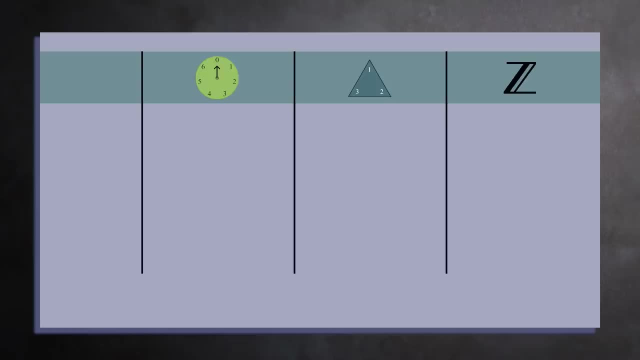 There are two other important properties these examples all share. For every element, there's an opposite element, which we call the inverse. For the integers under addition, the inverse of 3 is negative 3. The inverse of 7 is negative 7, and so on. And if you add an element and its inverse, you get 0, the identity element. For the symmetries, each transformation has an opposite as well. For example, the inverse of the element r that rotates 120 degrees clockwise is the transformation that's a double rotation, which is r squared. 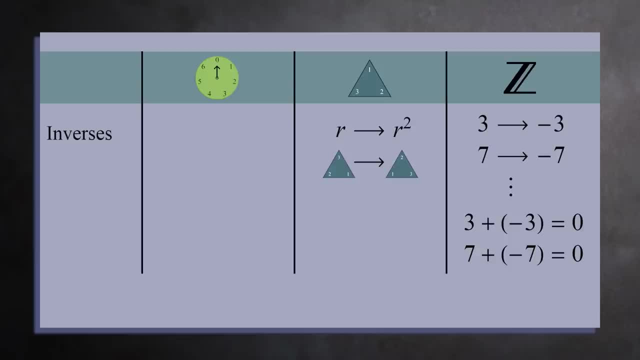 This is because doing three rotations makes a complete circle, returning you to the starting position. 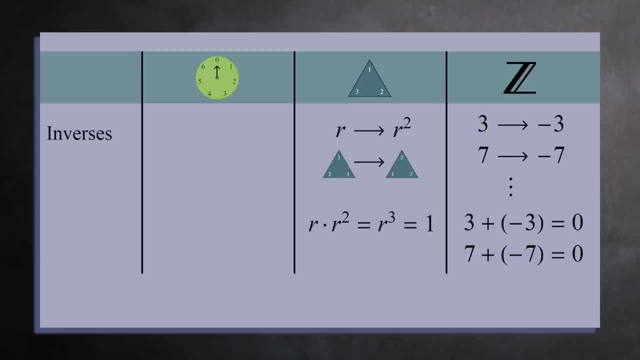 In other words, if you multiply r and r squared, you get 1, the identity element for the symmetries. 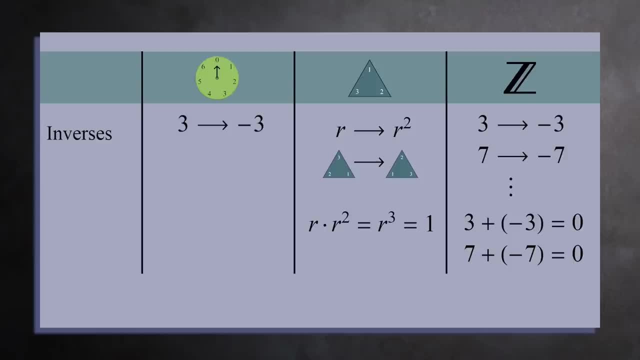 For the integers mod 7, the inverse of 3 is negative 3. But negative 3 is just 4 on the clock, so we say the inverse of 3 is 4. And 3 plus 4 equals 0, the identity element. 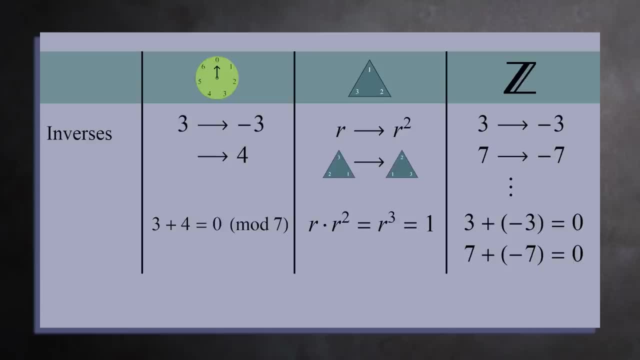 So for all three examples, each element x has an inverse. If you're using the plus sign for your operation, the inverse is written as negative x. 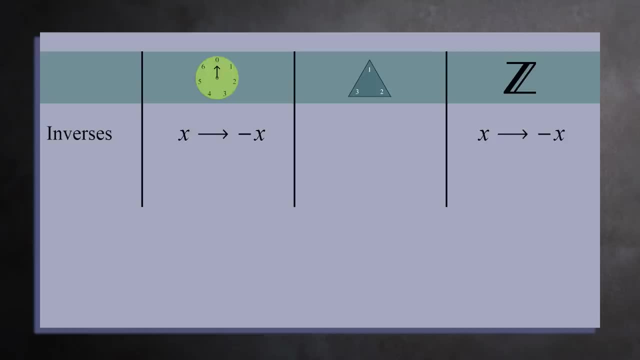 And if you're using the multiplication sign for your operation, the inverse is written as x squared. So you get x to the negative 1. Combining x with its inverse gives you the identity element. There's one final property that's essential in the definition of a group. That's the associative property. This just says that when combining three elements, it doesn't matter how you group them. You can start by combining the first two elements, or you can start with the last two elements. Either way, you'll end up with the same answer. 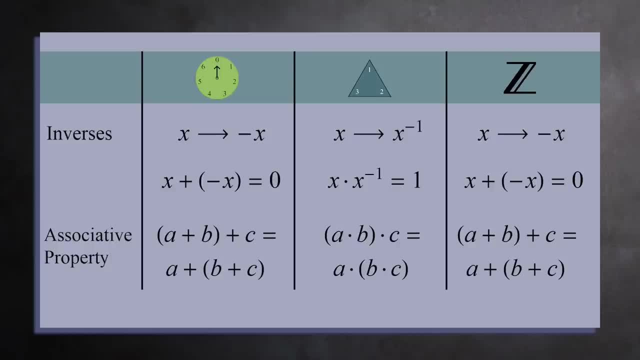 This is one of those properties people take for granted, but it's important nonetheless. 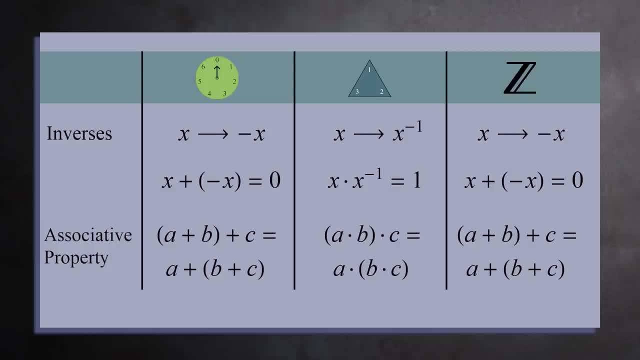 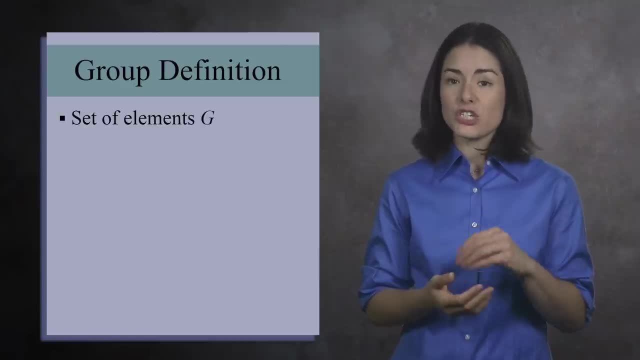 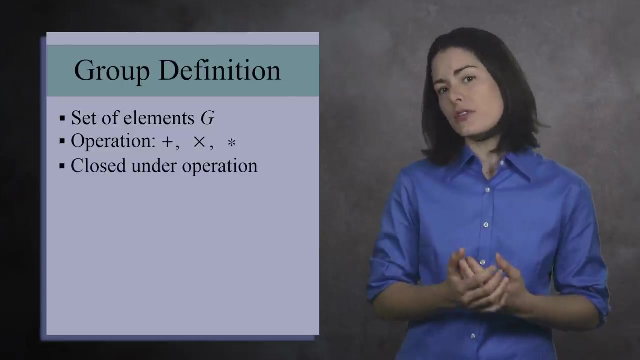 If grouping did make a difference, much of mathematics would come to a screeching halt. Let's now give the general definition of a group. A group is a set of elements G. It has an operation which allows you to combine any two elements. Common symbols for the operation are the plus sign or multiplication sign. But when speaking generally, we'll use an asterisk. Next, the group is closed under this operation. This means if you combine any two elements in the group, you get another element in the group. 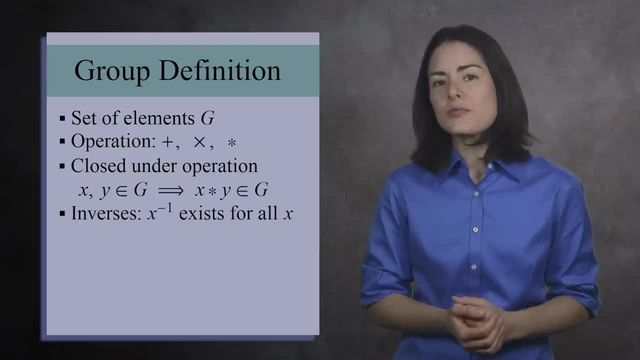 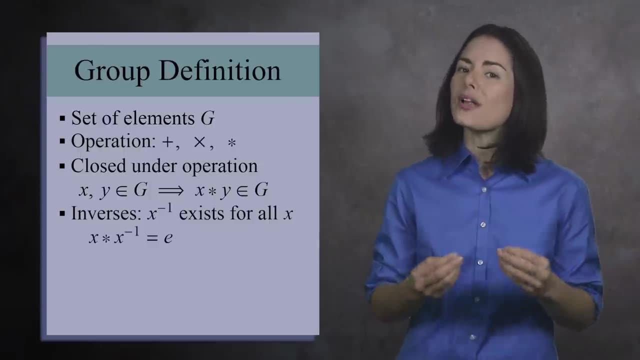 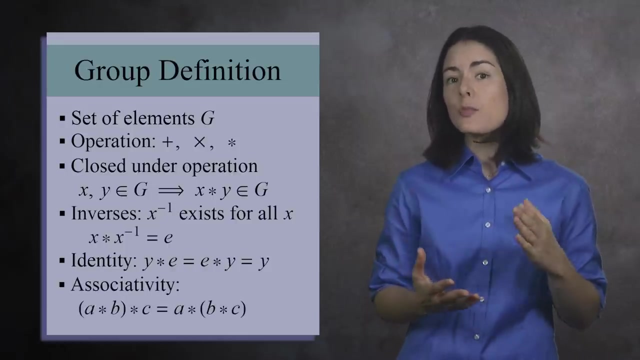 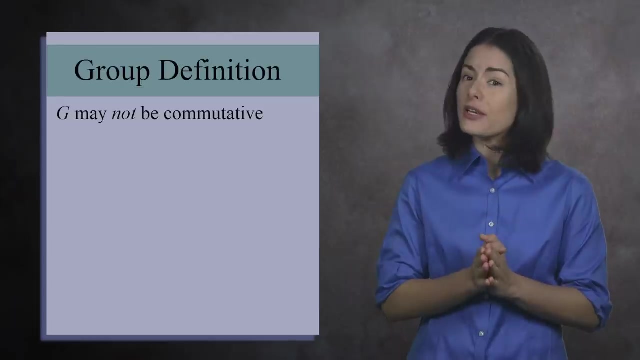 Each element X has an inverse. This is an object that has the opposite effect of X. And when you combine X and its inverse, you get the identity element, which we'll call E. If you combine any element Y with the identity element E, you get Y. And finally, the elements obey the associative property. This is the definition of a group. It took mathematicians many years of work to identify these as the most essential properties. For example, notice that groups are not required to be commutative.